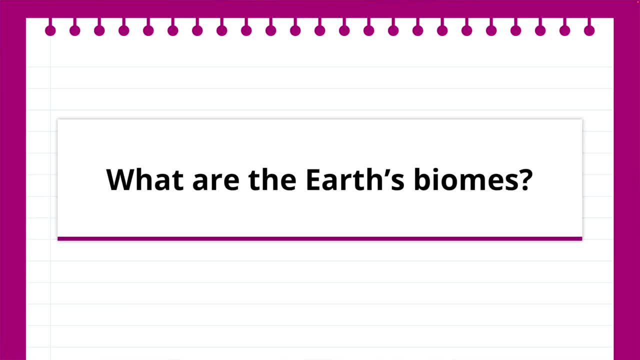 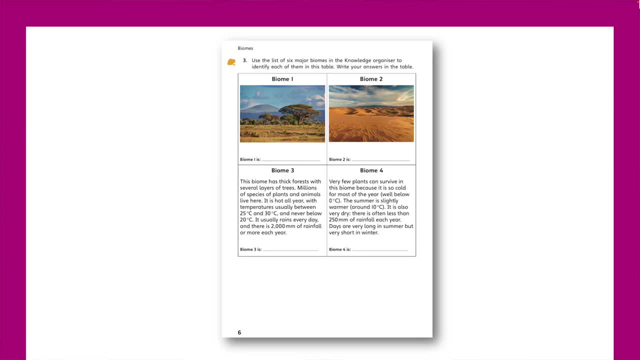 The first lesson asks: what are the Earth's biomes? Pupils will learn the names, locations and key features of six biomes before having a chance to apply this knowledge by identifying biomes through pictures. This is an activity that can be easily extended, and the more 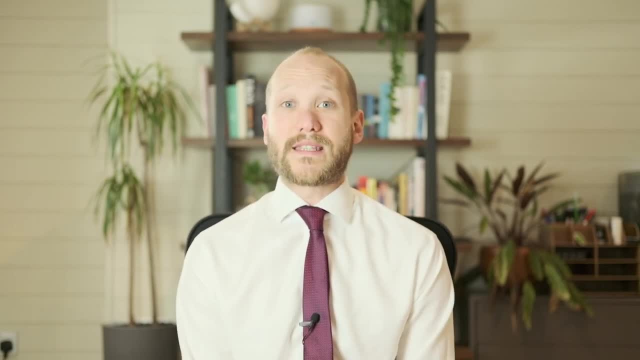 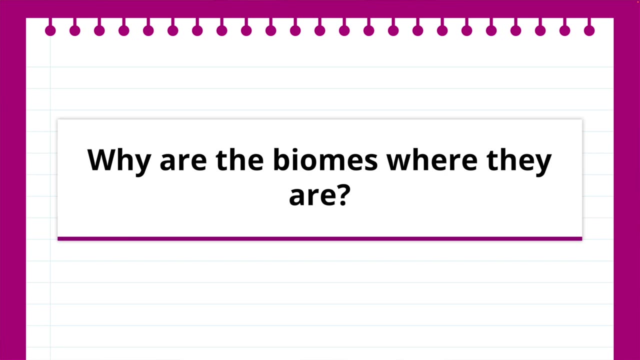 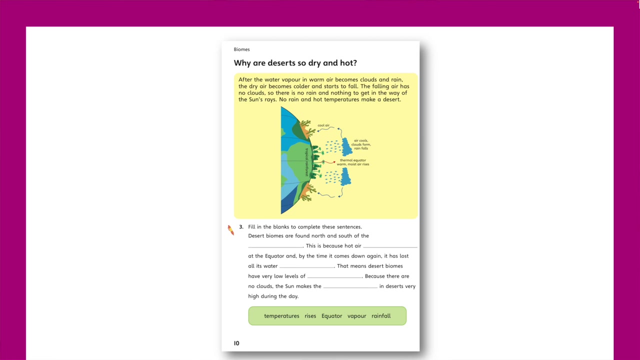 visual examples, pupils have a chance to explore the stronger sense they will have around what each biome is. Lesson two asks: why are the biomes where they are? This lesson allows pupils to get a good sense of location, especially with regard to lines of latitude and how different. 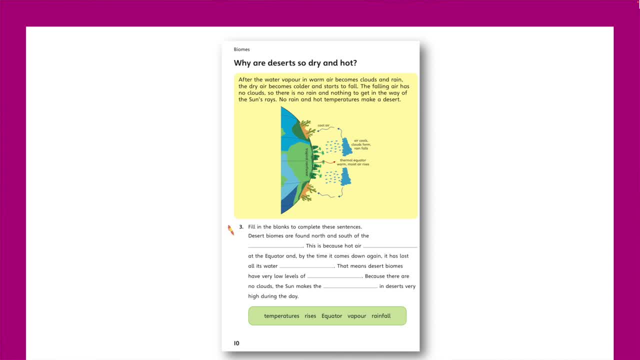 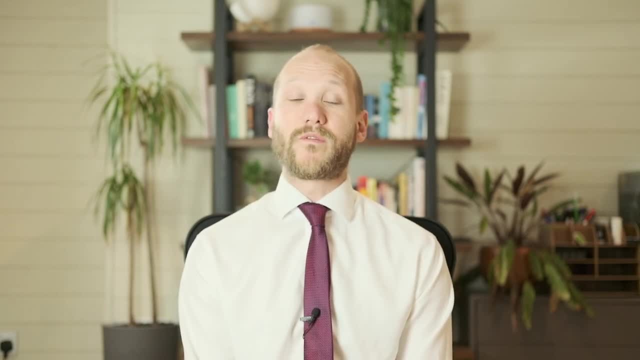 parts of the world experience different climates as a result of where they are located. They will learn about the tropical zones close to the equator, and temperate zones as we move further north or south. Finally, the polar zones, which receive almost no direct 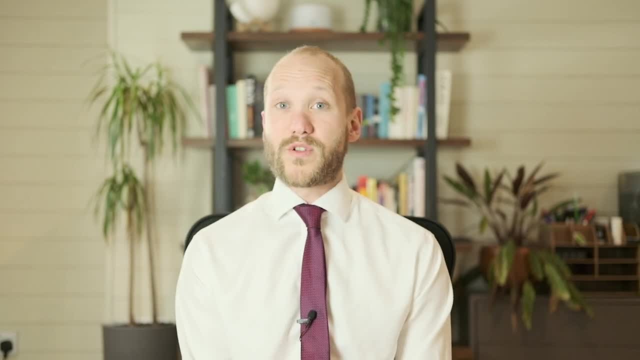 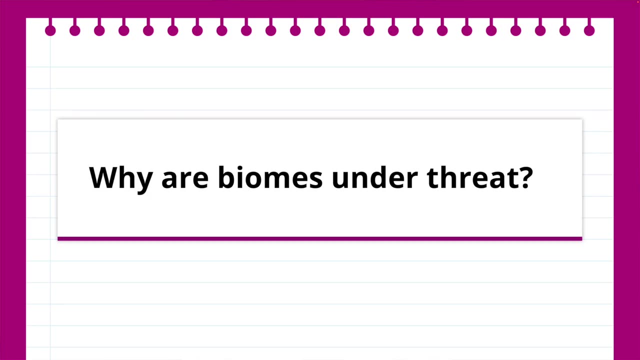 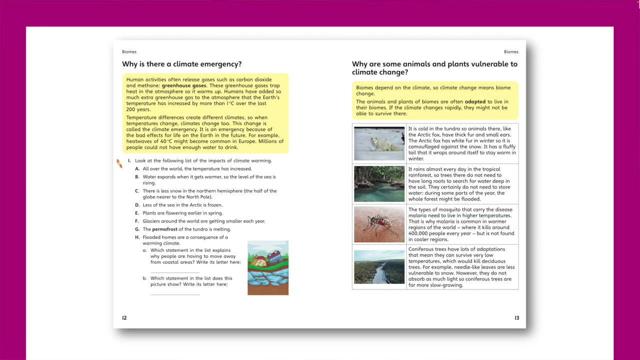 sunlight will be located. There are lots of great opportunities to link this knowledge with science lessons. Lesson three asks: why are biomes under threat? In this lesson, as pupils consider the causes and impact of the climate emergency, especially with reference to flora and fauna which live. 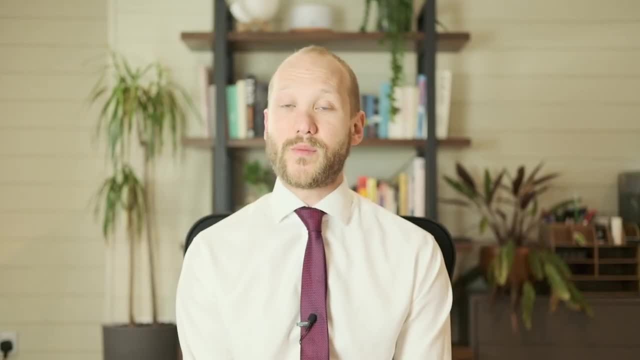 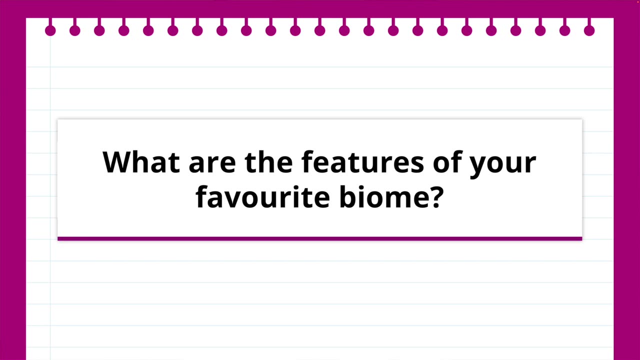 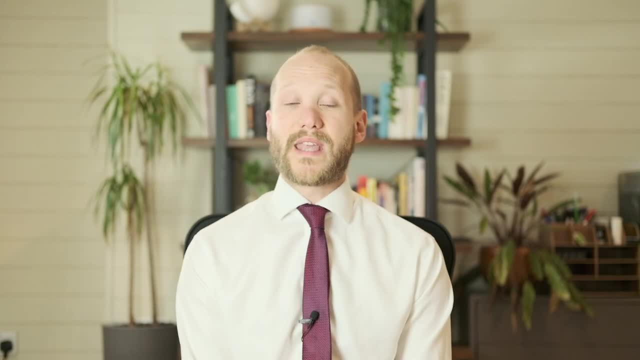 features of your favourite biome. Here we will explore the features of your favourite biome. Here we will explore the features of your favourite biome. Here at może, pupils will have an opportunity to engage in much more depth in their favourite biome, as well as. 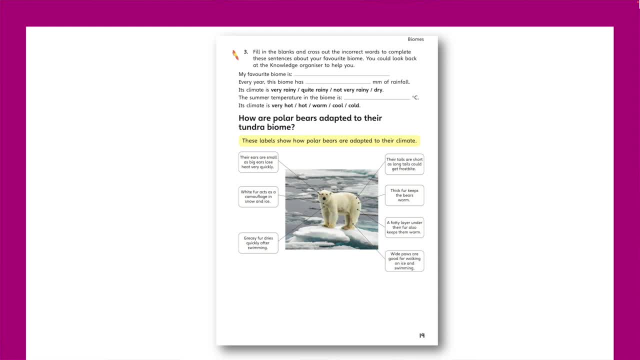 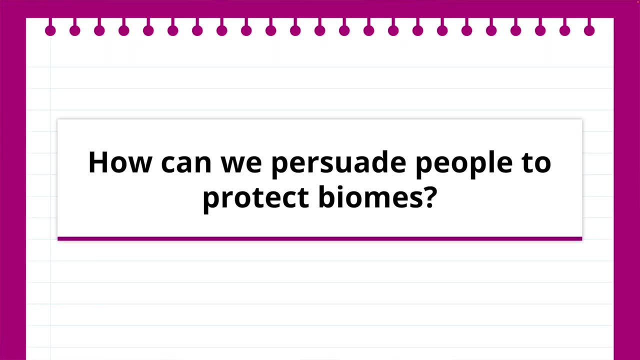 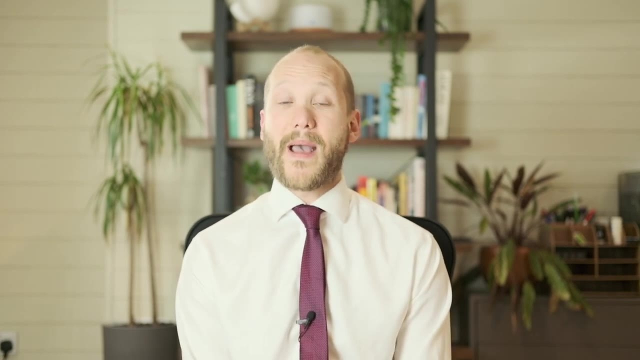 how the flora and fauna of the region have adapted to the climate and conditions there. Lesson five asks how can we persuade pupils to protect biomes? When learning about the impact of climate change to the flora and fauna of different biomes, pupils often feel a very passionate sense of responsibility. This lesson will 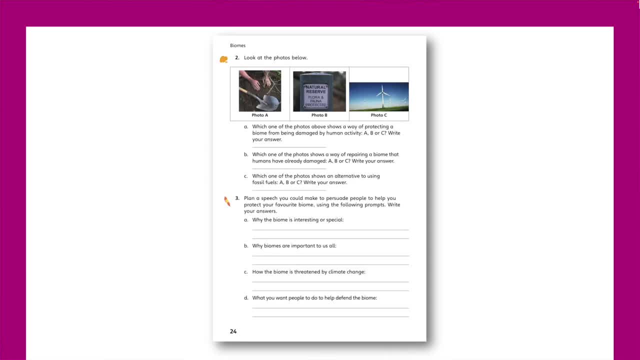 direct pupils towards writing a speech to set out kinds of milhões and models for mouth-or-v Frostongerasia. Here you will learn some useful ges, Narratives of which can help studyzeded articles, books to set out the challenges and potential solutions for protecting biomes. And the final lesson.